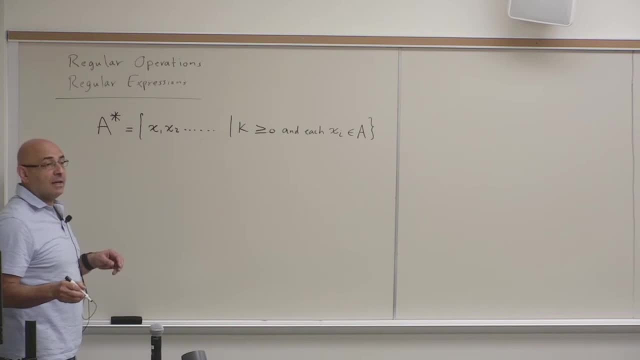 that the string can be of infinite length. A string cannot be of infinite length. A string must have a finite length, but the length is unlimited. So this is a subtle point: Each string, each valid string, has a finite length, But the length of a string is not limited. 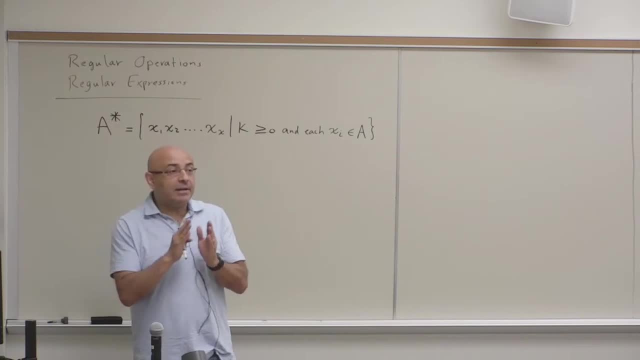 So you can accept an arbitrarily long string, Which means, which then implies, that the number of strings that you will have in this language is infinite, Because you are not setting a limit on the string length. Each length, each string, has a finite length. 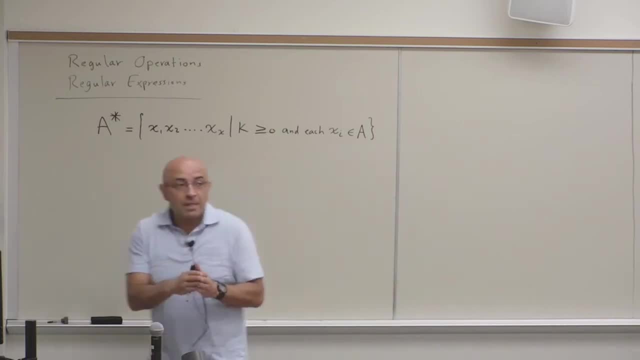 But you are not setting a limit on the length of that string To make it, you know, more concrete and related to actual programming and compilers In compilers. how do you use this in compilers, In fact, as you will see when we later talk about compilers? 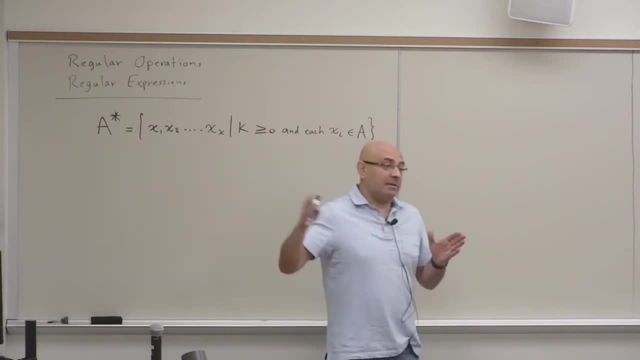 the compiler is going to view the whole program as a string, no matter how long. So if you have a program that consists of millions of lines of code, the compiler is going to view it as a string of characters. Now, the compiler can process a program only. 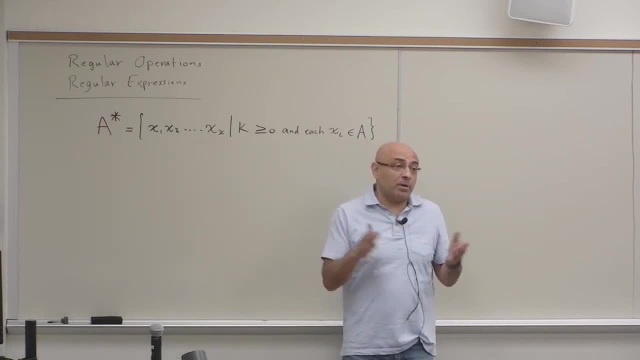 if that program has a finite length. In fact, there is no problem. You cannot write a program that has an infinite length Because you'll have to write it. So any program that is written by human beings within the lifetime of a human being, it's going. 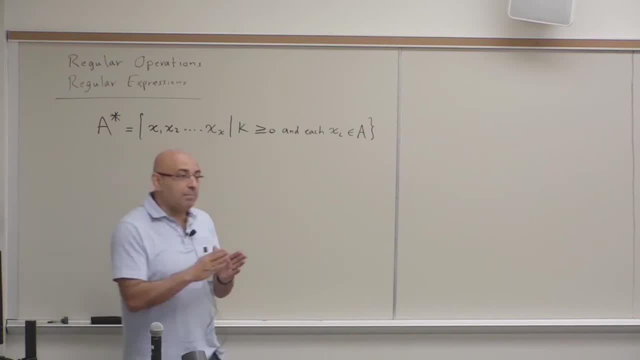 to have finite length. So the compiler can process a program, processes programs with finite lengths, But there is no limit on the length of that program. So did you ever try to compile a program, a very long program, with a compiler, and the compiler said: 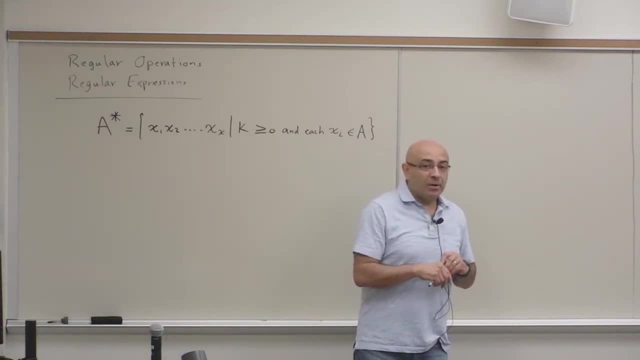 this program is too long for me to compile. No, The compilers that I'm aware of do not have this limitation. At least you know the algorithms, the compiler algorithms. There may be some limitation on the resources. I mean the compiler is trying to compile a program. 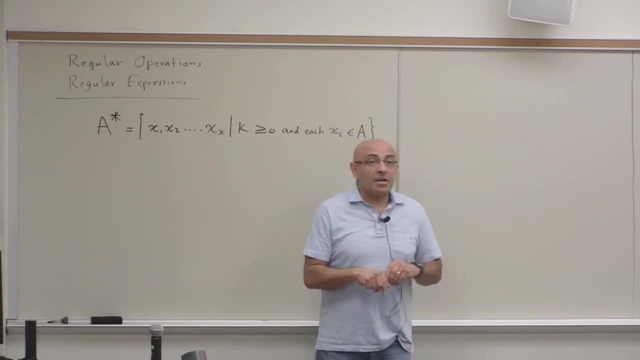 that is too large. It may exhaust system resources like memory or whatever, but that's a different story. You know the compiler itself, the algorithms in the compiler are designed to accept an arbitrarily long program. So this is the idea, the right definition of this. 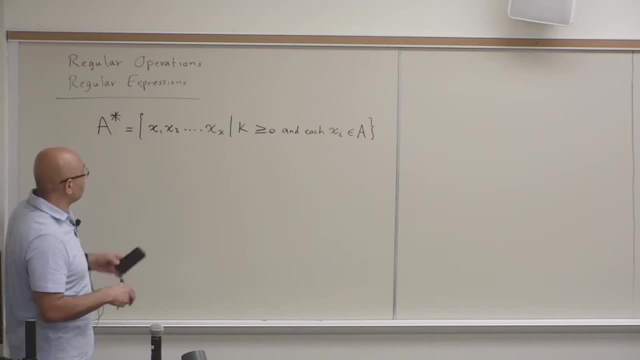 the algorithm. So this is the idea of the star operation And it's important to pay attention to these subtleties. Now let's review regular expressions by giving a couple of examples on regular expressions before we move to the main topic of today's lecture. 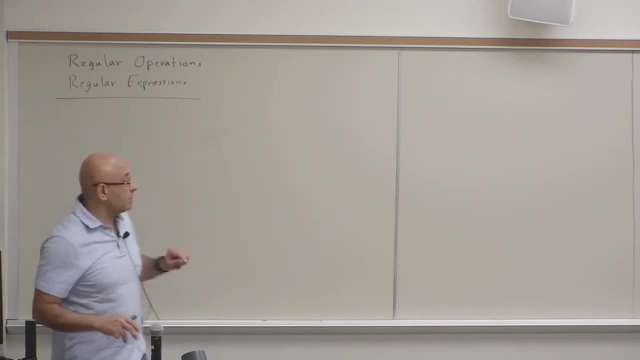 which is closure properties of regular language. So let me give you this Last time. you know, we gave the language and then you know, I asked you to figure out the regular expression. Now I give you the regular expression and I ask you to figure out the language. 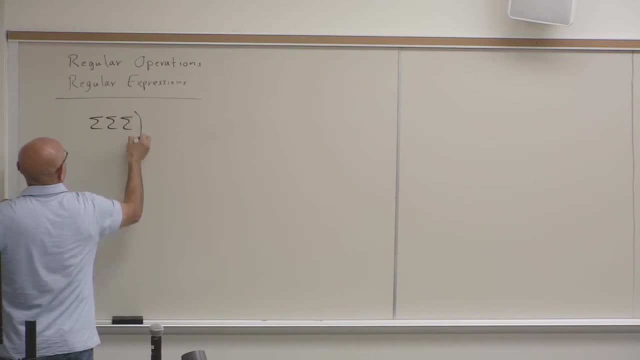 What about this regular expression? Of course, you know, remember: sigma is any one symbol and sigma star is any. what? Any string, Any string Including, Yeah, any string Including the empty string. Okay, Now, what language does this regular expression generate? 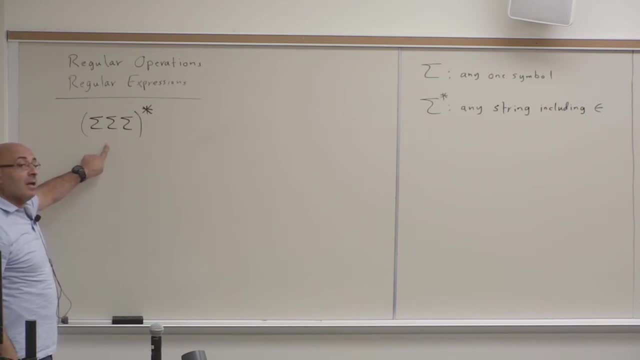 Multiple of three. Multiple of three. Okay, What's the multiple of three? So give me a more precise description of the language. What should be? what quantity should be a multiple of three? N, Three, What quantity? The length of the string. 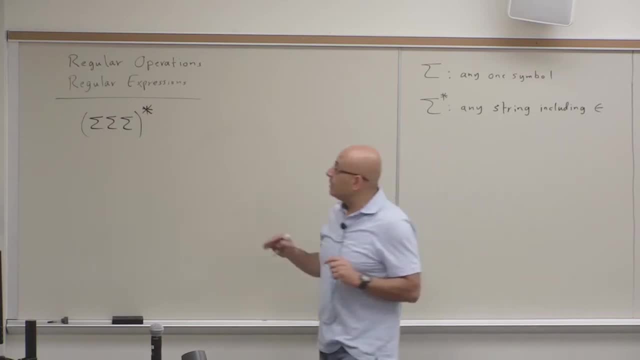 The length of the string is the quantity that is, a multiple of three. So we have to be specific L. we have to be precise here. W is the set of strings W such that the length of W is a multiple. a set of strings W such that the length of W is a multiple. 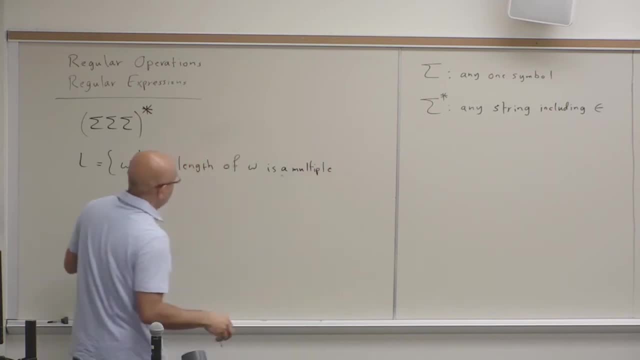 a multiple of three. By the way, if you write something like W, such that W is a multiple of three, this is not. this is incorrect, because W is a string. It's not a quantity. It's not a number. W is a string, not a number. 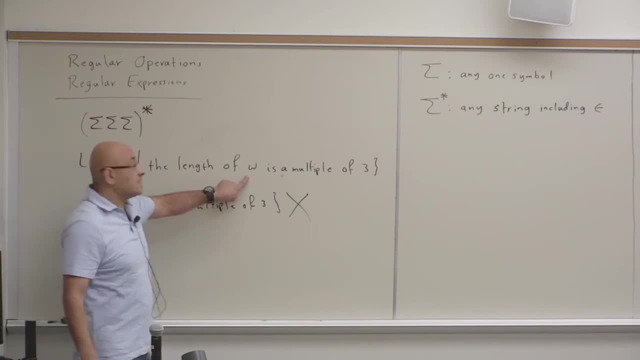 The length of W is a number, It's a quantity, It's a multiple of three. Okay, So in language description we have to be very precise. Okay So, we figured this out. So let me give you this: I like three. 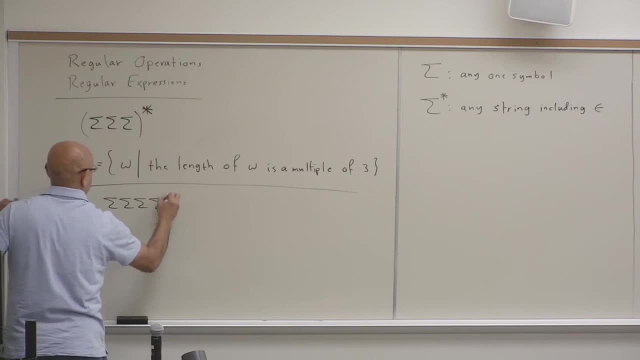 So let's do this. So what's the language here That is generated by this? It has at least three symbols. Yeah, It's the set of strings that consists of three or more symbols, Or the length of the string that belongs to this language is greater than. 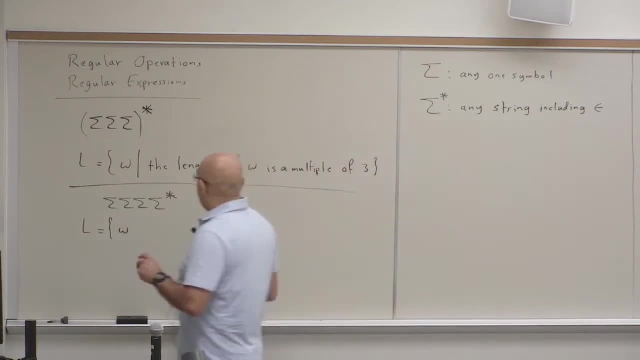 or equal to three. Okay, So, such that the length of W of W is greater than or equal to three, Or another way of saying it, W consists of three or more symbols. These are two different ways of describing the language, but both are precise and clear. 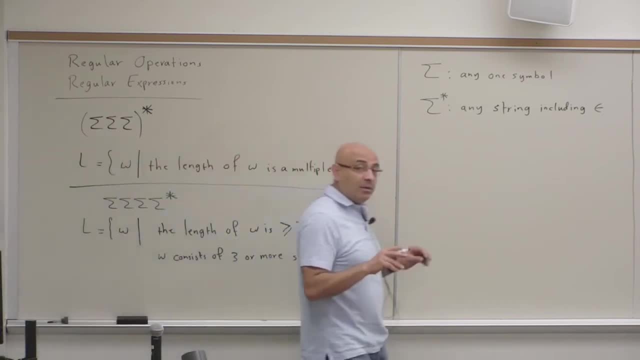 But make sure that when you say that something is greater than three or less than three, you're talking about a quantity or a number. Okay, So these are two examples just to refresh your memory. Let's now give some examples of languages and try to figure. 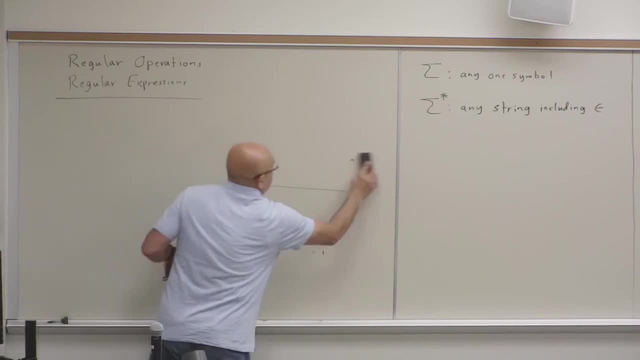 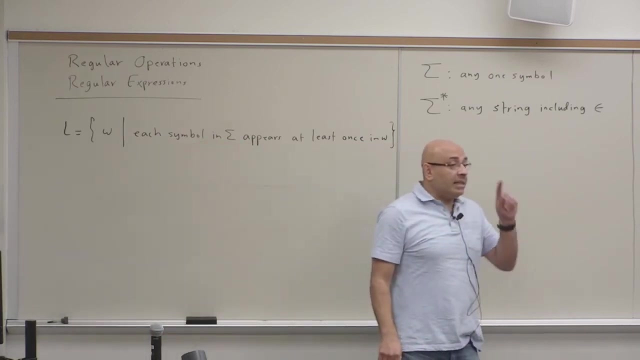 out the regular expressions. Okay, A language W, such that each symbol in sigma appears at least once in W. W is a string in which each symbol in the alphabet appears at least once, Or another way of saying it is that there is at least one occurrence. 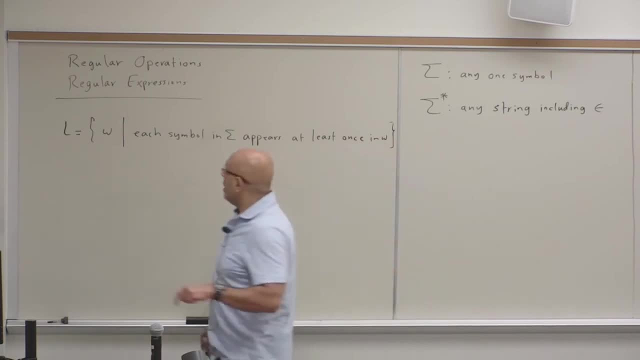 of every symbol in the alphabet. There is at least one occurrence of every symbol in the alphabet. Okay, Now, of course, we cannot answer this question without knowing what the alphabet is. So the alphabet here is going to be AB. Now for this alphabet. how would you write a regular expression for this? 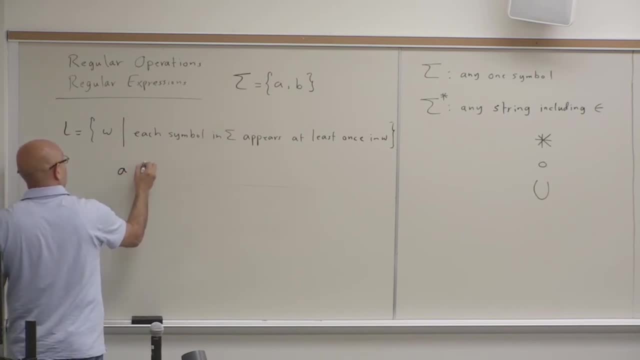 Okay, So we have AB, right, and Sigma stars. Yeah, sigma stars, yeah. Sorry, it's my fault. Don't you also need an OR? Because what if B comes before A? Sorry, I was thinking of something else. 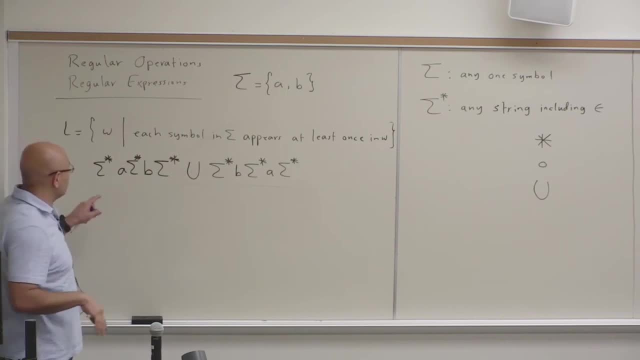 So that? yeah, so thank you for the question. Yeah, so it's AB, and you know before, after, between, you can have anything, And B, then A, you can have anything. Now, what about this W, such that W starts and ends with the same symbol? 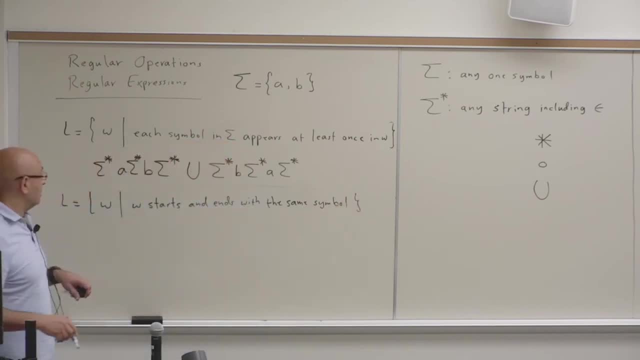 W starts and ends with the same symbol. How would you do this? What's the regular expression for this? You would have A, then any symbol start, any symbol start, and then B, or, and then you just have the mirror image of that. 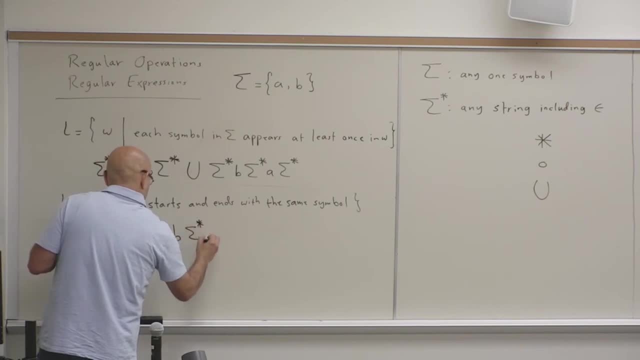 So B- any image, start, A What starts and ends with the same symbol. Oh no, I meant I should have said A starts, then A, or B- any symbol, B. Yeah, Professor, I think you said A. 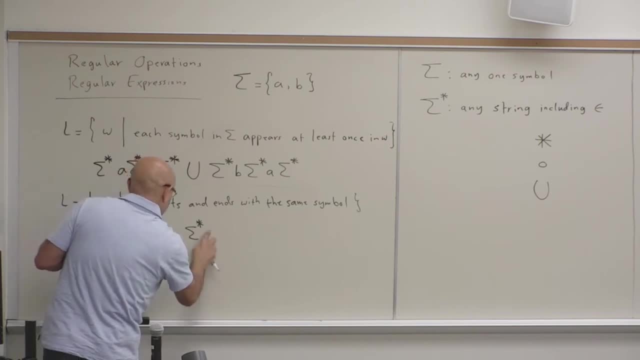 but I screwed up? I think No, I totally said the wrong thing. Okay, okay, So it starts and ends with the same symbol: A segment start A. B segment start B. So if you give this answer in the test, 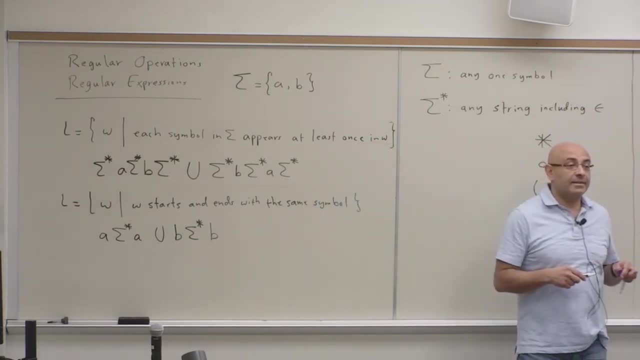 you will get 9 out of 10 or 8 out of 10.. Why? Because it's missing something. What is it missing? It's not covering all the strings that satisfy this problem. What's that? It's blank. No, blank doesn't start and end with the same symbol. 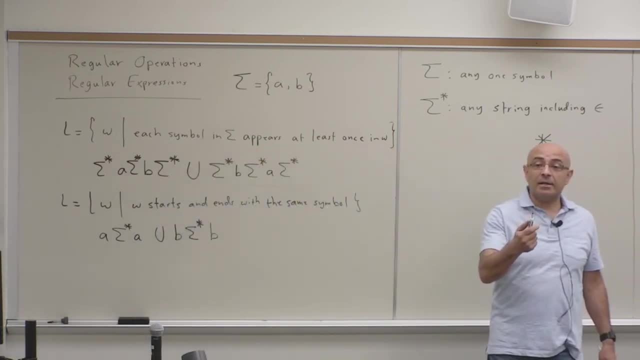 Yeah, yes, anyone. What should we add? What's that? Epsilon doesn't start and end with the same symbol because it doesn't even start. It doesn't start at all. So what are the strings that start and end with the same symbol but are not covered by this? 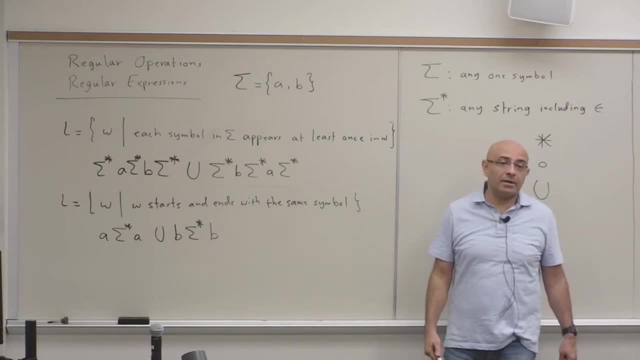 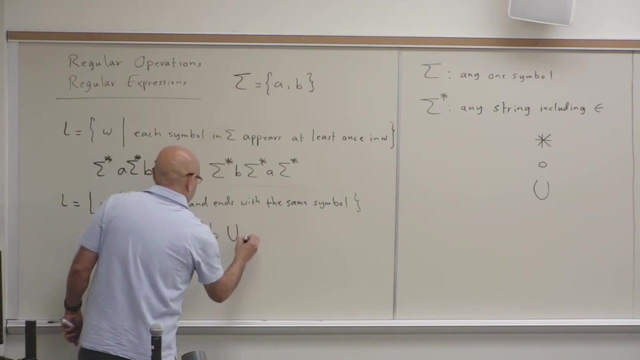 The strings of length 1.. Yeah, the strings of length 1. A by itself or B by itself. So make sure that you cover all the corner cases. So here you have A by itself or B by itself. Okay, so this is a corner case. 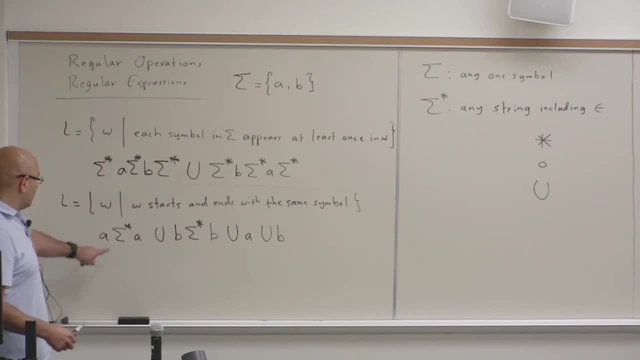 or a special case that you need to cover. So this is the strings that are of length 2 or greater, that start and end with the same symbol, Start and end with the same symbol of length 2 or greater, And this is the string with one symbol that starts. 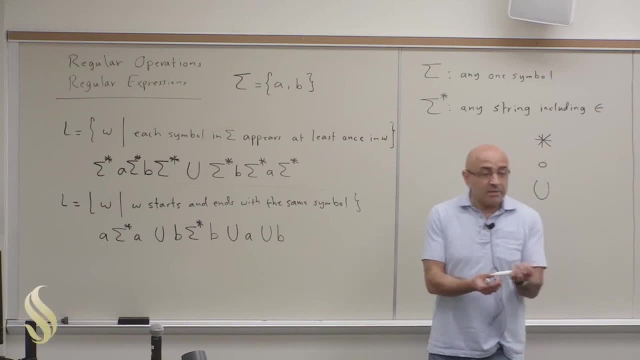 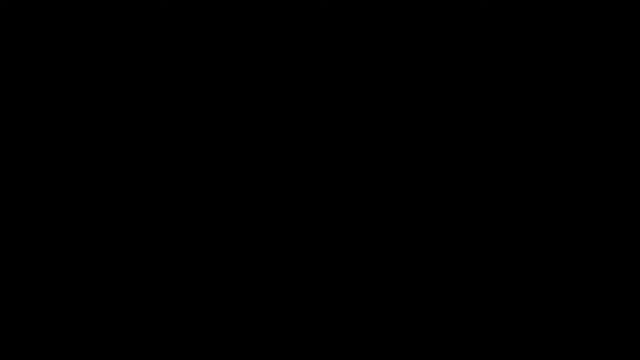 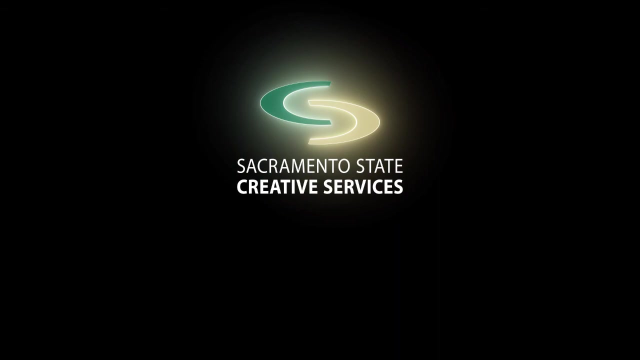 and ends with the same symbol. Okay, so I think we have enough examples now to clarify the idea of the regular expressions, And I think now we are ready to do the homework. Thank you.